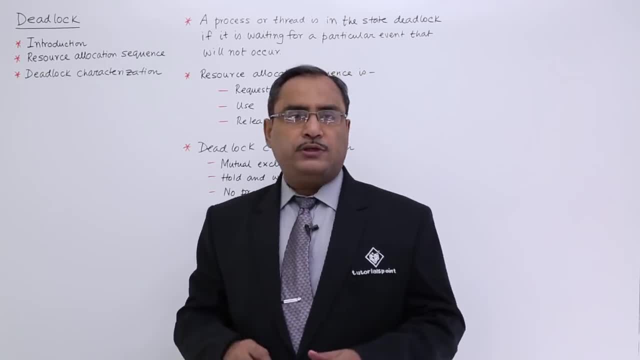 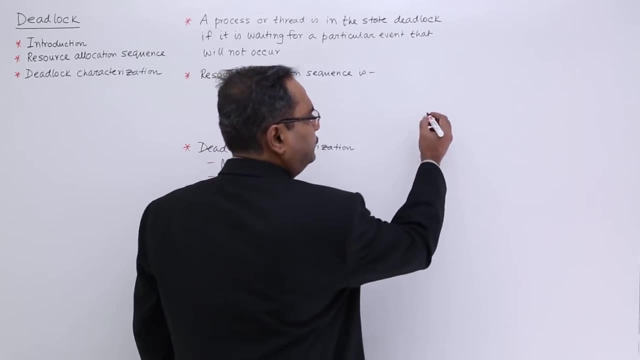 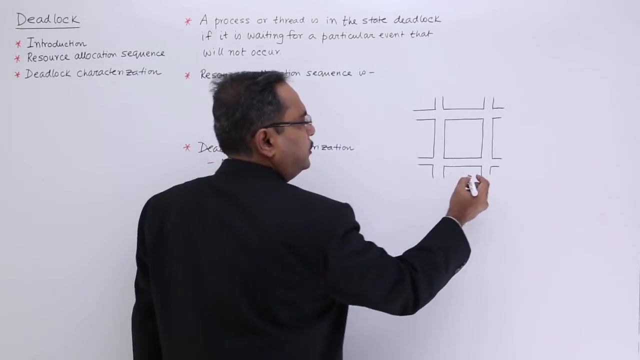 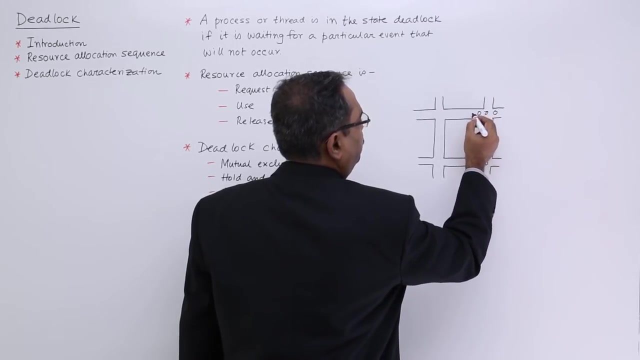 and then deadlock characterization. So these are the topics we are going to cover in this particular session. So we know that if we have, say, a road like this, So some cars are trying to move in this direction, some cars are trying to move in this direction, some. 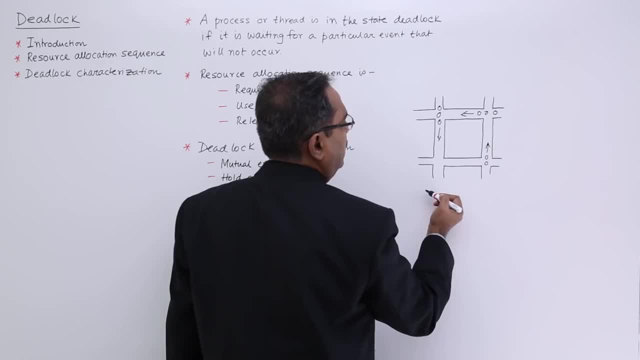 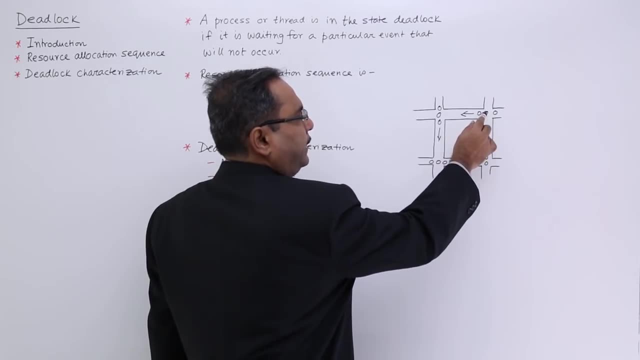 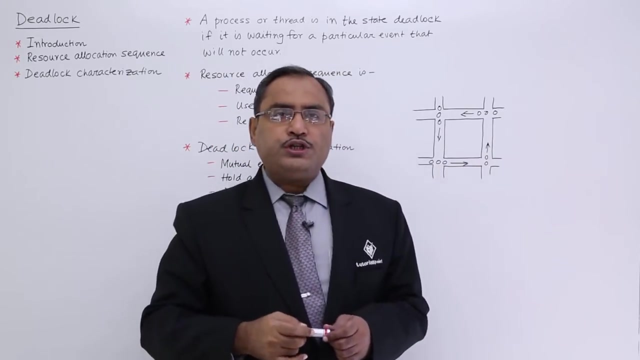 cars are trying to move in this direction, and some cars are trying to move in this direction. Then what will happen? You see, they are getting blocked by them, they are getting blocked by them, they are getting blocked by them and they are getting blocked by them. So what will happen? A congestion? 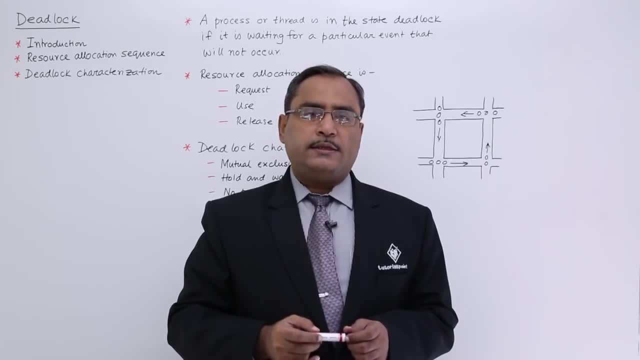 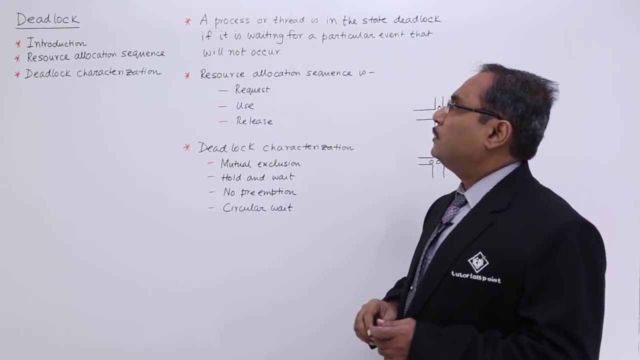 will take place and that congestion is known as a deadlock. So in operating system a deadlock can be defined in this way: a process or thread that is in the state deadlock if it is waiting for a particular event that will not occur. 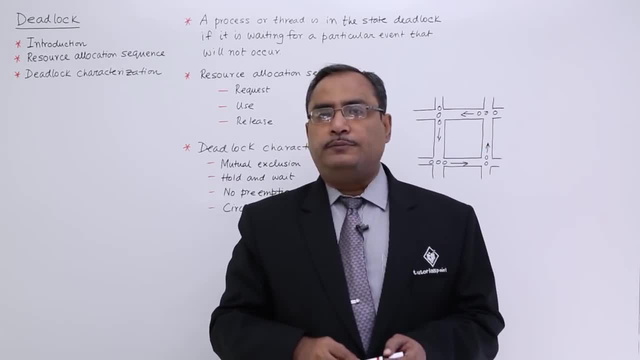 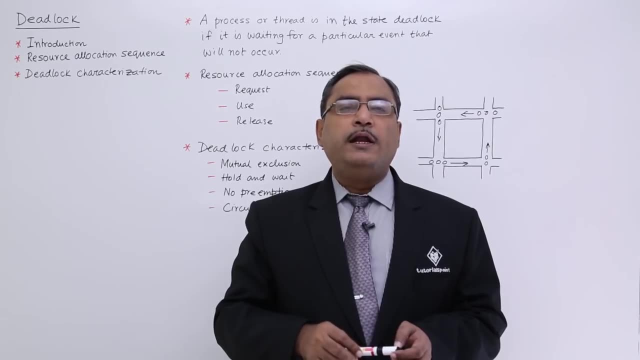 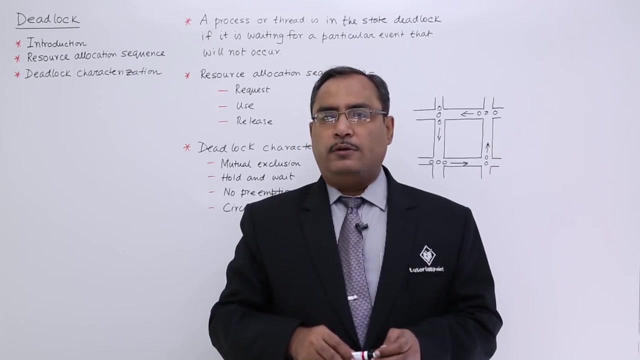 So that is the definition of a deadlock. So that means a process. its progress has been blocked due to the unavailability of the resources or due to some other incidences, and that is the situation of occurrence of a deadlock. When deadlock occurs, then you: 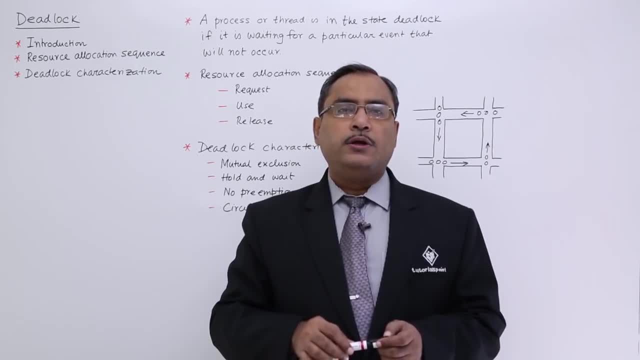 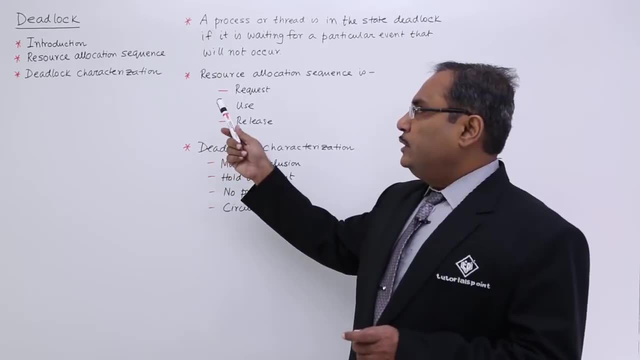 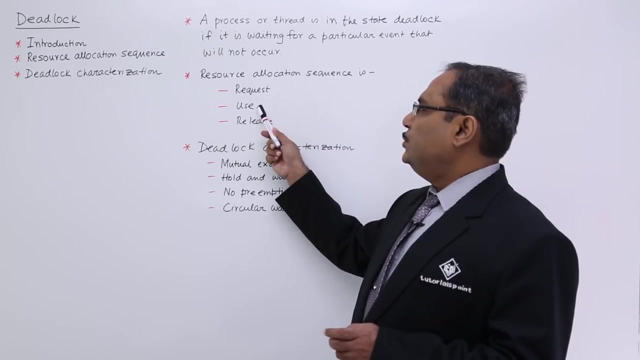 should execute some deadlock recovery routine to retrieve the system from the deadlock situation. So let me discuss one by one. So now we are going to discuss what is the resource allocation sequence. The resource allocation sequence is request, use and release: request, use and release. 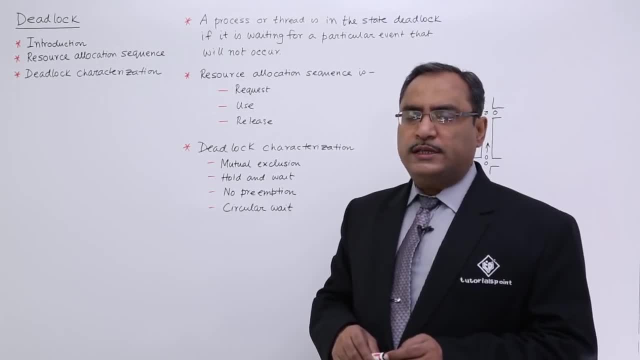 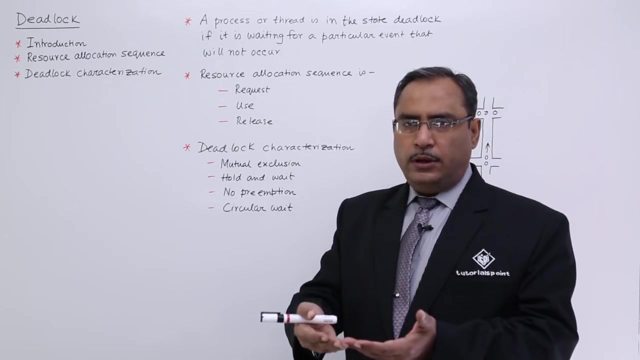 What is request? In this particular case, the process will place a request to the operating system to grant one of the instances of a particular resource to the process. So request means the process will place a request to the operating system to grant one of the instances. that means at least the resource should be available to the process. so it 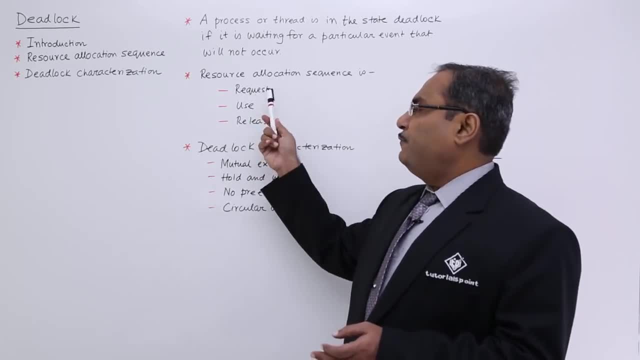 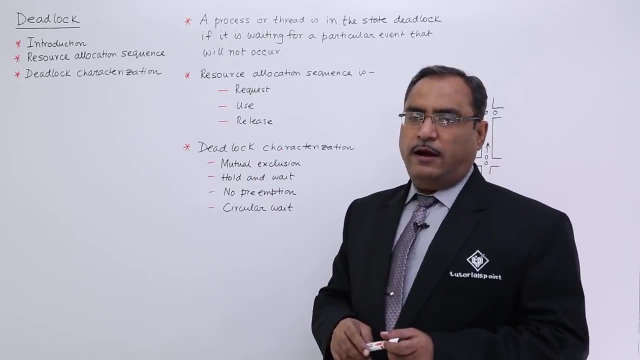 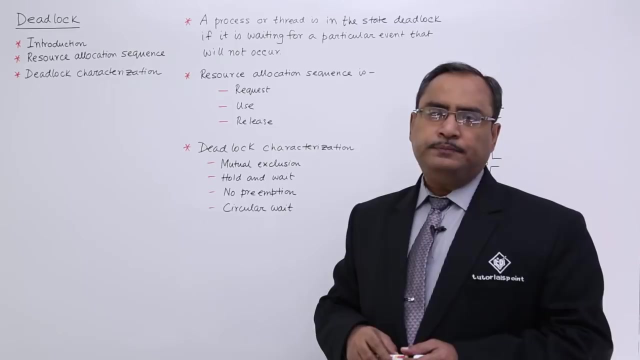 will place a request to the operating system. If operating system grants the request, then the process will be in a state to use the resource and after completion of the usage of that particular resource, the process will release the resource and that will be going for the other process. 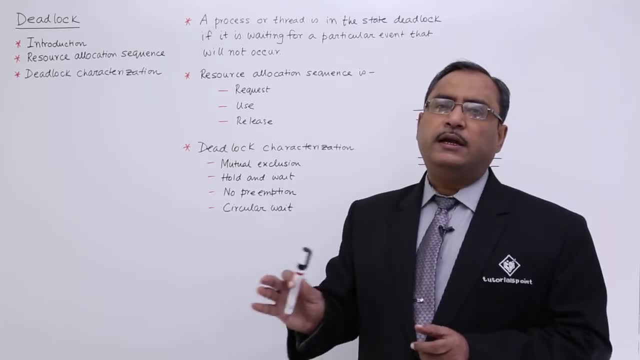 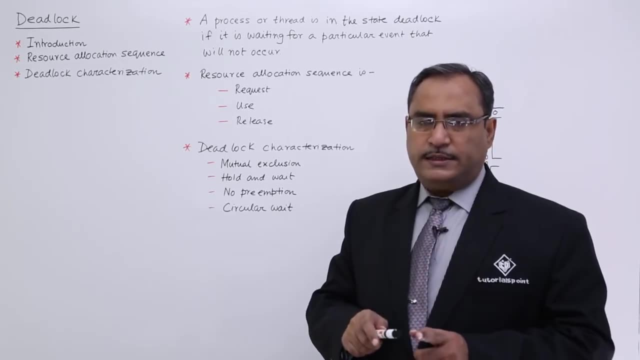 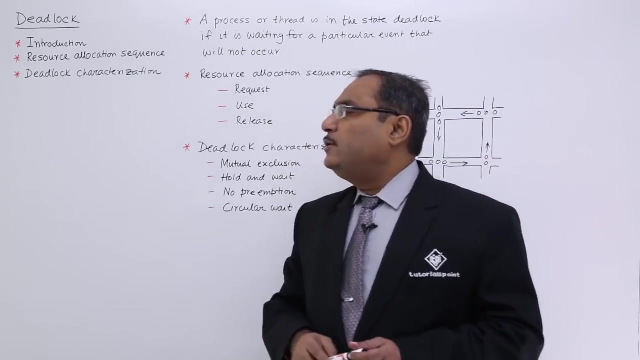 Other processes to get access over the resource if they are requesting for it. so request, use and release. So these are the three different sections through which a resource can be allocated to a process. My next agenda topic is deadlock: characterization, deadlock- why deadlock happens. The deadlock happens mainly for this, mainly for this. four reasons: One is a mutual exclusion Deadlock, Deadlock. What is mutual exclusion? That means at a time a resource can be allocated to a single process. If it is so, that means if the resource is non-shareable, then the probability of occurrence 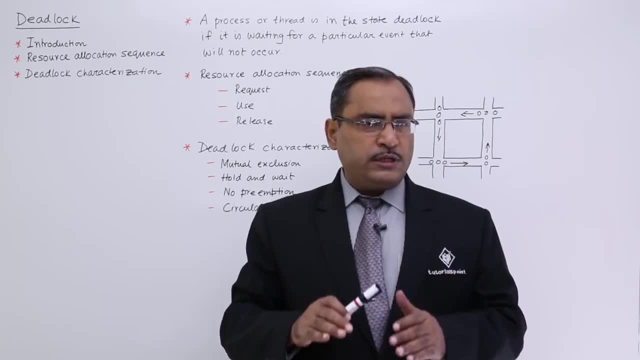 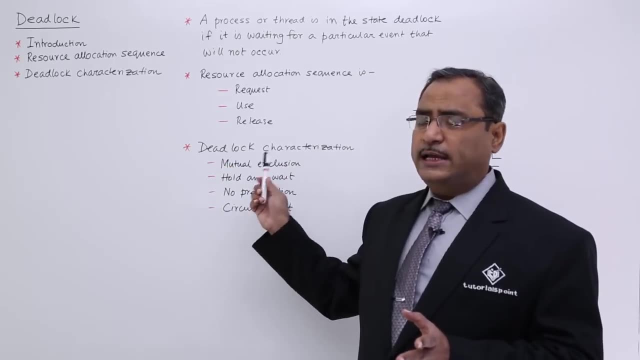 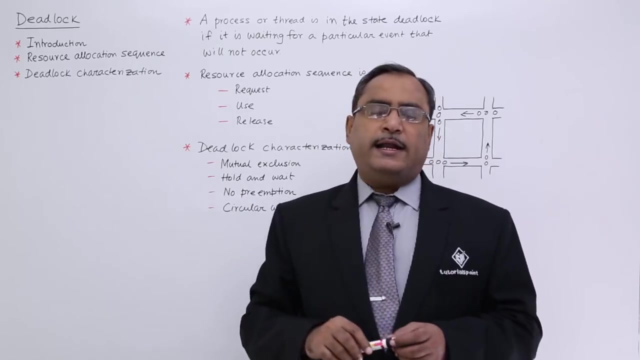 of deadlock will get increased. But if the resources are shareable at the same time, if a resource can be allocated to multiple processes existing or executing in the system, then obviously the deadlock probability will get decreased. So mutual exclusion means at a time the resource can be allocated to a single process. 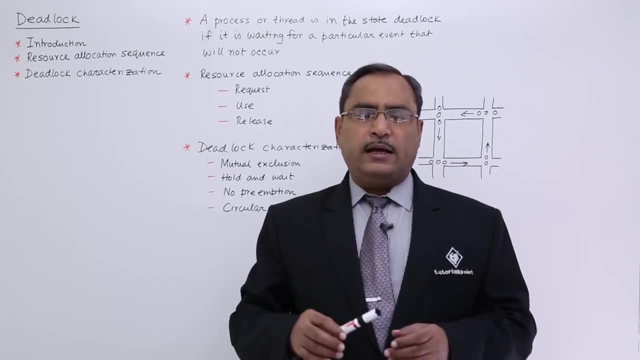 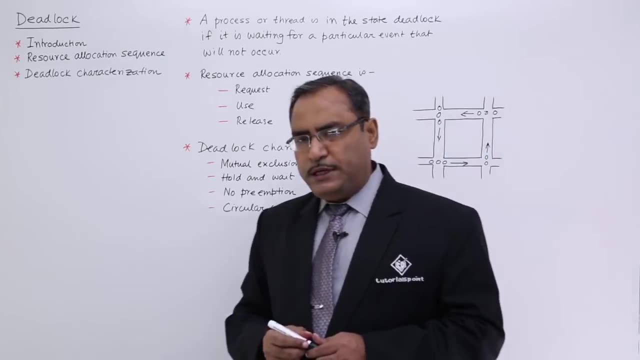 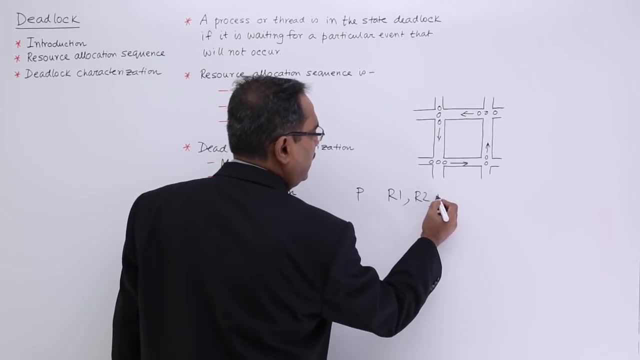 If it is so, that will go for the increase in the probability of occurrence of deadlock. Next one is hold and wait. Say that is one process P which is requiring three resources. Say one process P which is requiring three resources. say R 1,, R 2 and R 3.. 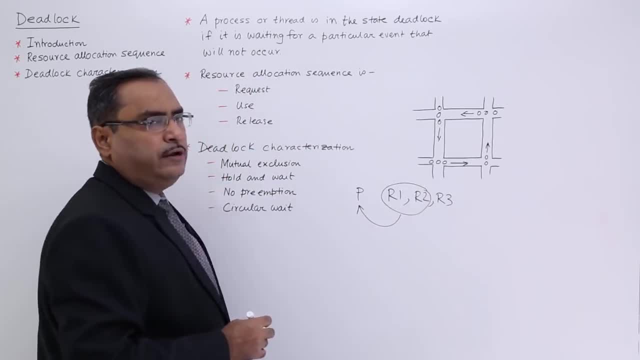 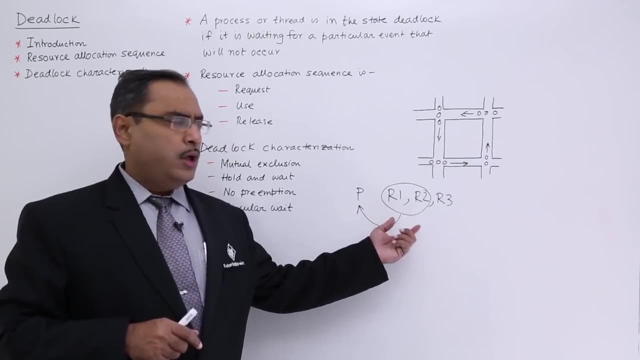 Say R 1 and R 2 have got allocated to P and P is waiting for R 3. And if P waits for indefinite period of time holding these resources- R 1, R 2- and waiting for P hold and wait, then that will be one of the causes of occurrence of deadlock. 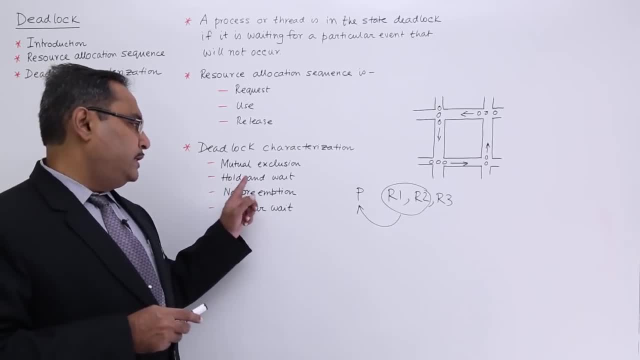 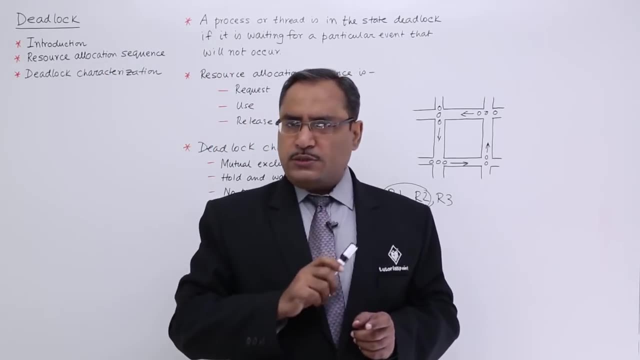 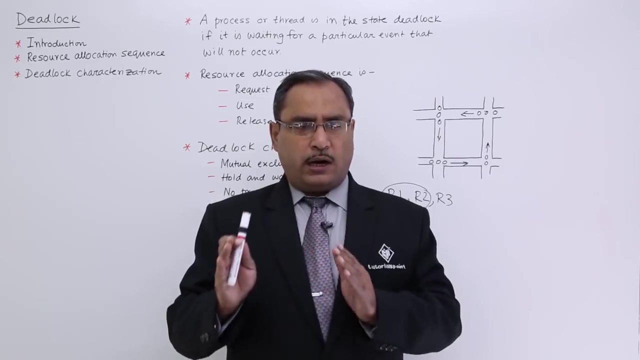 So this name is the causes hold and wait. Next one is no preemption. That means voluntarily: a process will not release any resource until completion. That means, let us suppose, a process is occupying R 1,, R 2,, R 3.. 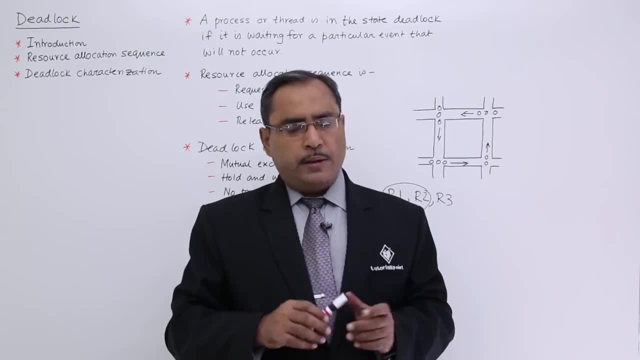 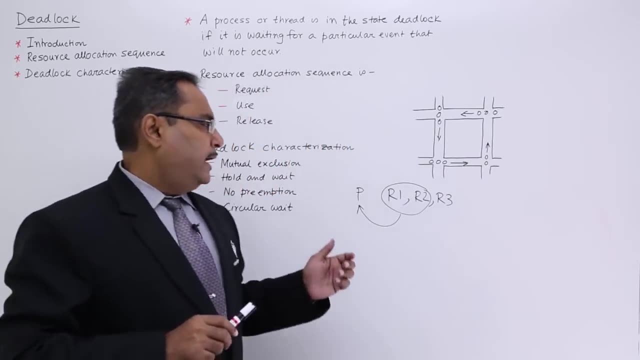 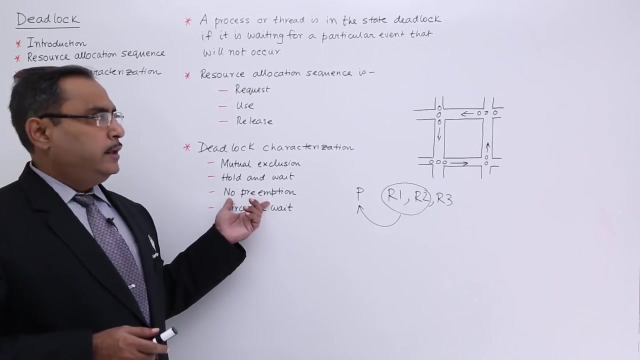 But the job or task with R 1 has got completed by the process P but the process P will not release the resource R 1 until it gets completion. then that might be one of the probable causes of occurrence of deadlock and that is known as no preemption. 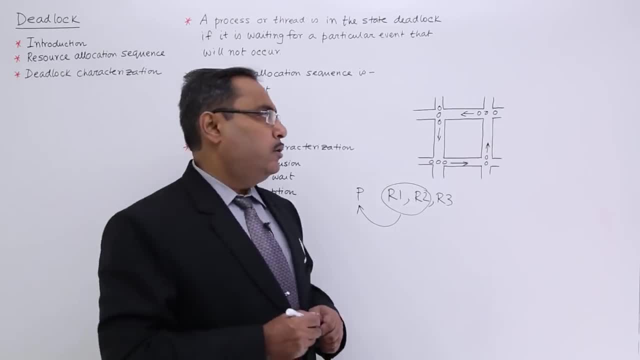 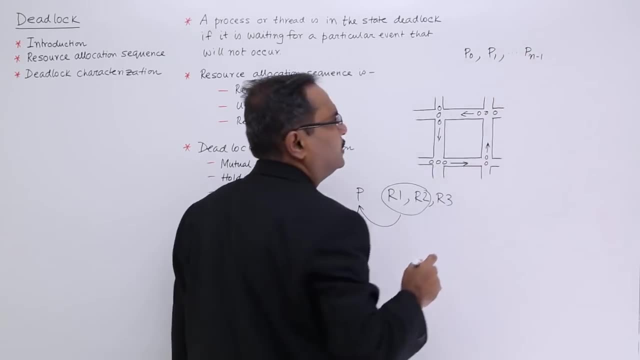 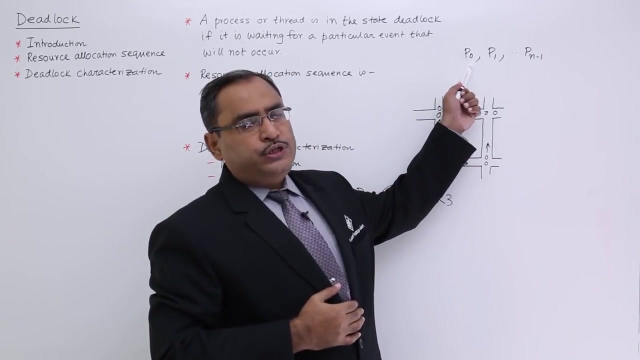 The last one is my circular wait. What is circular wait? Say we are having P 0, P 1, dot dot dot, P n minus 1 processes. So how many processes are there? N number of processes. Good, Let us suppose P 0 is holding a resource which is being required by P 1, P 1 is holding a